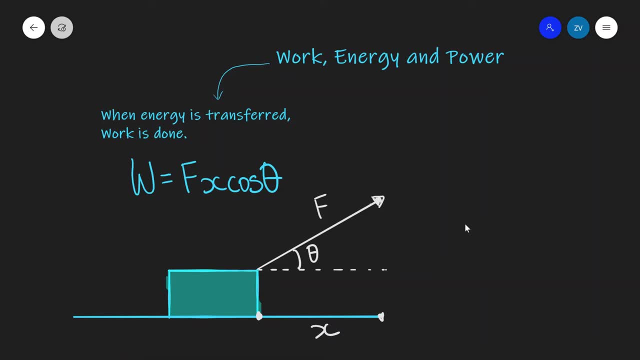 Hello everyone, welcome back to Zed physics. Today we're going to be revising work, energy and power. I'm going to be following the OCR physics A specification. however: as always, the physics is applicable to all exam boards. So let's get started Now. what is work done? Work done is. 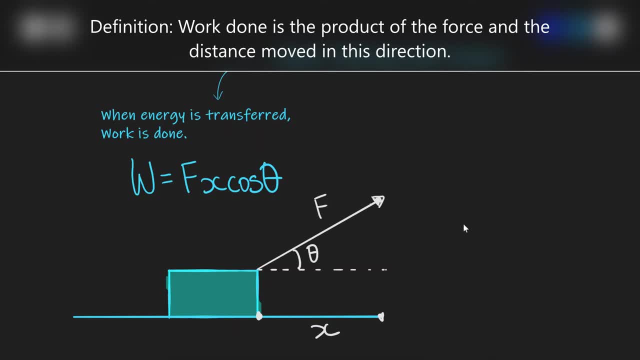 defined as the product of the force and the distance that's been moved in its direction. The formula, the A-level physics formula for work done, is that work done is equal to fx cosine of theta. In this equation, f is the force, x is the distance that's been traveled and theta 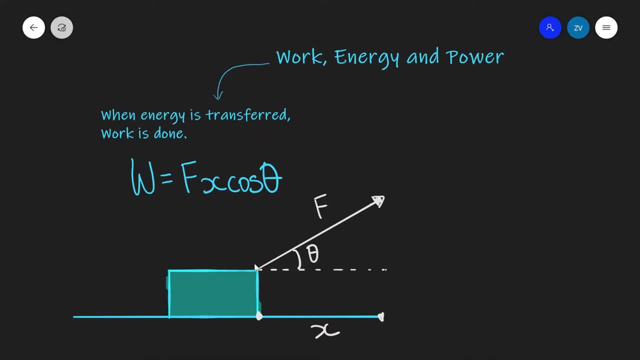 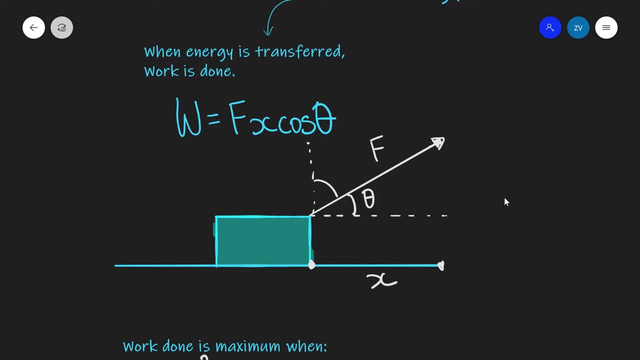 is this angle here? it's the angle between the force and the displacement of the object. It is very important to note once again that theta is the angle between the force and the direction of the displacement. Occasionally, in a question, they might try and trick us by. 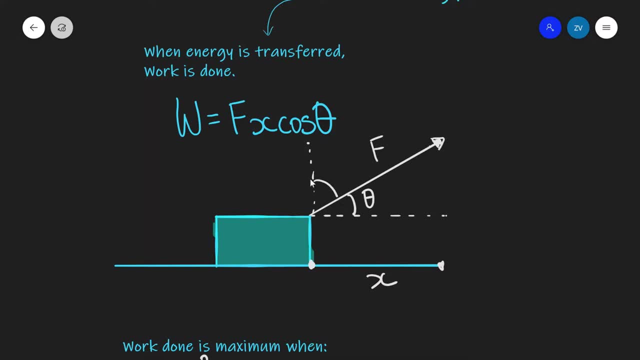 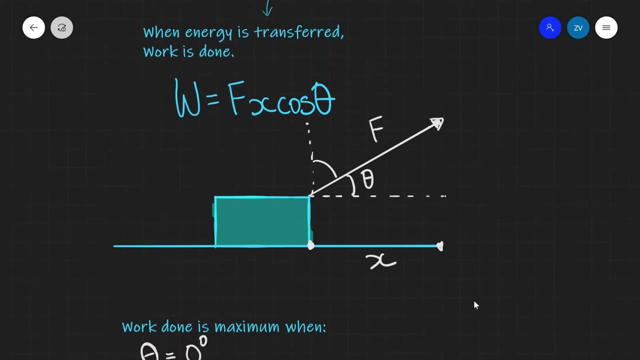 giving us this angle here, and if that's the case, we need to subtract it from 90 to get theta. Okay, now that we know what work done is, when is work done? a maximum, The maximum work done, happens when your angle theta is equal to zero degrees. 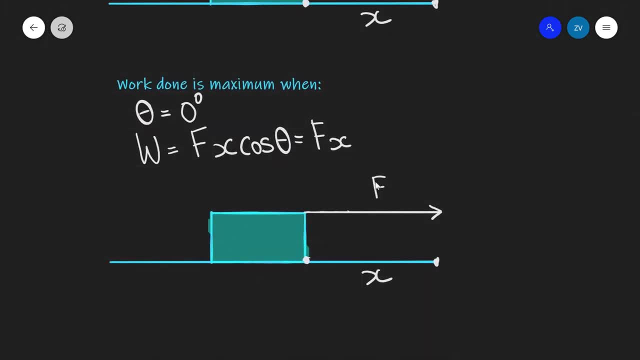 If theta is equal to zero degrees, then your angle theta is equal to zero degrees. If theta is equal to zero degrees, then your angle theta is equal to zero degrees. So when you have two sides and the force is interconnected, this means that your angle 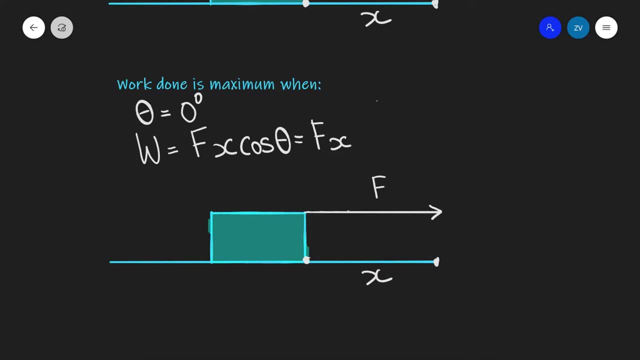 theta is inbspair for one term in your correct form. So if theta is inspair for one term and your angle theta is inspair for one term, then your angle theta is inspair for one term. in your 0.บ. speedane under 6 zero degrees, then your angle theta is in comic 0.ları. 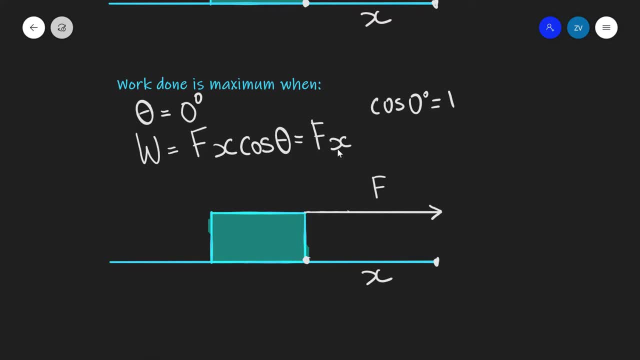 That's the case, that if theta is in the Bake Cow's curve, at least what's tstage. so we have T squared plus z, but that's not what's across the curve of the curve. So if theta is in this tipo of relationship, The outside angle comes out to equal that. 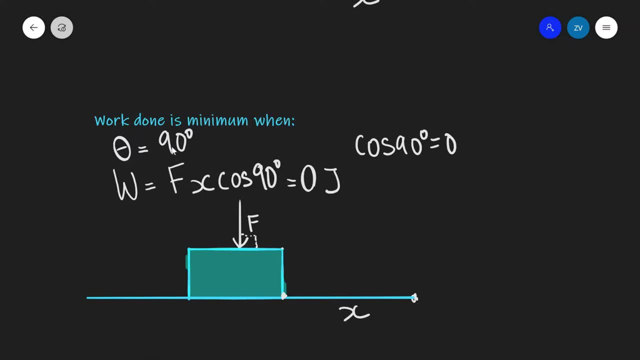 angle theta by t свое режim over y. your angle is 90 degrees. remember that cosine of 90 degrees is equal to zero, which means that work done being f times x times cosine of the angle, which in this case is 90 degrees, will. 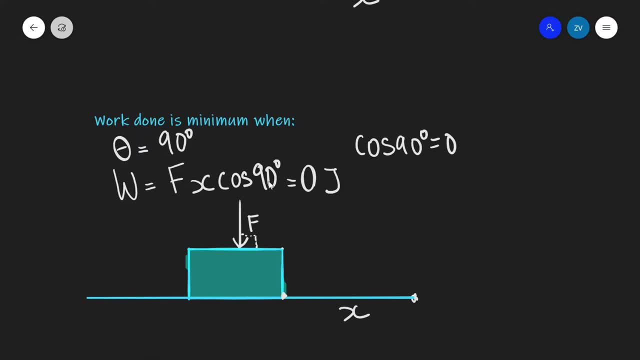 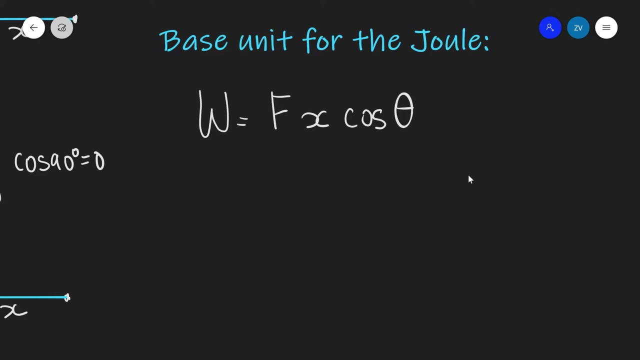 give us zero joules overall. So if we're applying a vertical force, there will be zero work done in the horizontal direction. We have just mentioned that the unit for work done is the joule, exactly same unit as the unit for energy. Now what is the base unit of the joule or the base unit of work? 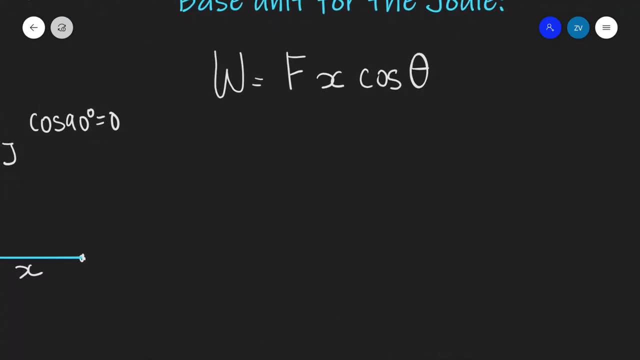 done. So we know work done is equal to f times x times cosine of theta. Now the force is given by mA, so another way of writing the following equation would be mA times x times the cosine of theta. Now, in the following equation, mass is of course measured in kilograms. Acceleration is going to. 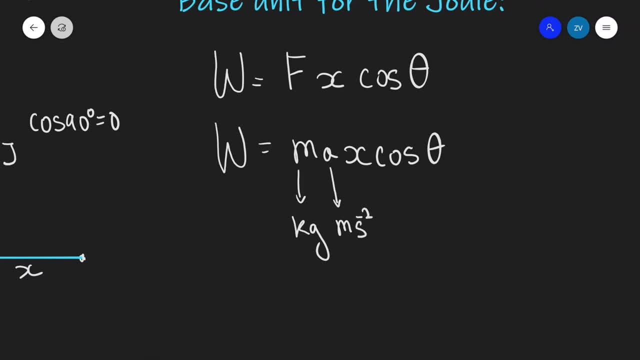 be measured in meters per second squared. so that's mS to the power of minus two. Our distance traveled is measured in meters And cosine of theta. well, this is unitless. In fact, all of the trigonomic functions have no units. I'm just going to make a little note here and I'm going to 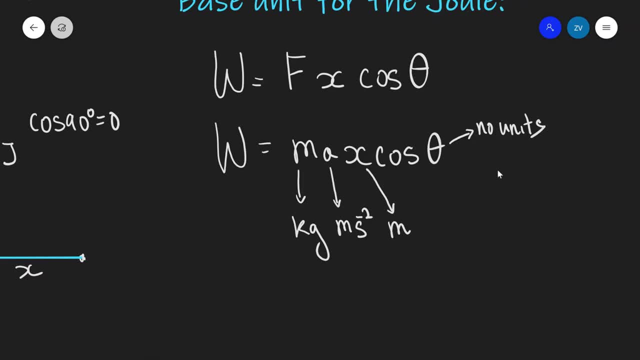 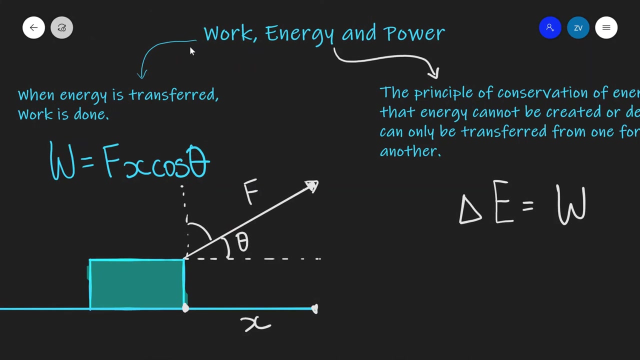 say no units. So the joule is actually equal to kg times meters S to the power of minus two times meters. again, Another way of writing this is just simply kilograms meters squared S to the power of minus two. Ok guys, now that we've looked at the work done, let's have a look how it actually connects with. 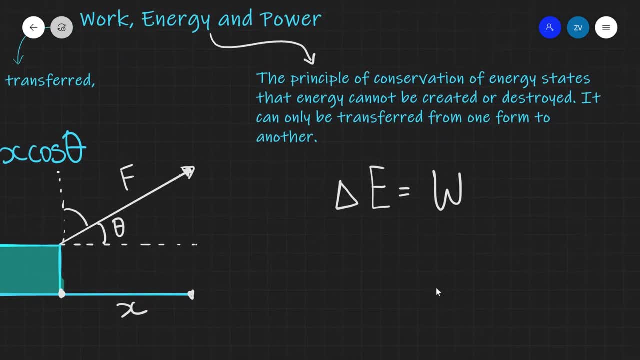 energy, of energy states that energy cannot be created or destroyed. it can only be transferred from one form to another. We're all familiar with the different types of energies. for instance, you can have kinetic energy or kinetic energy that's been transferred to, let's say, potential energy. 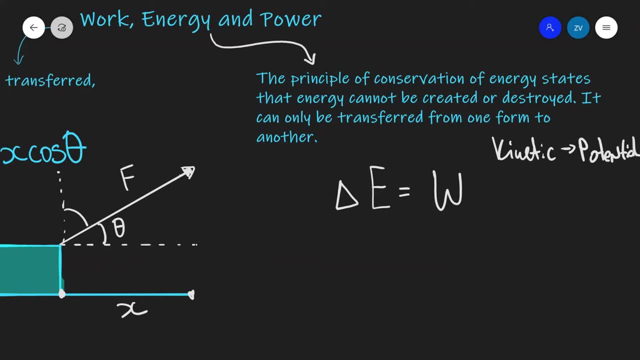 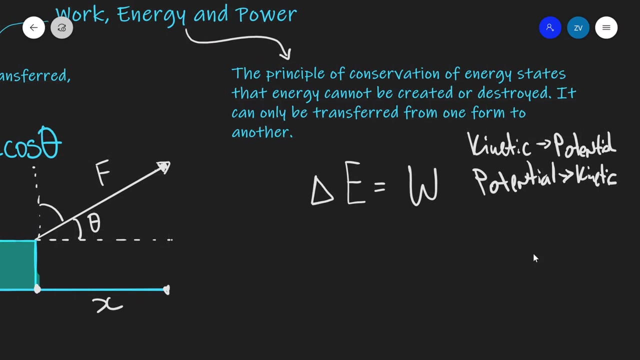 for, to throw a ball up in the air, or we could have potential back to kinetic energy when that ball falls to the ground. We could also have various different types of energies, such as thermal energy, nuclear energy, etc. Now, what we're going to be focusing on, though, is a very, very 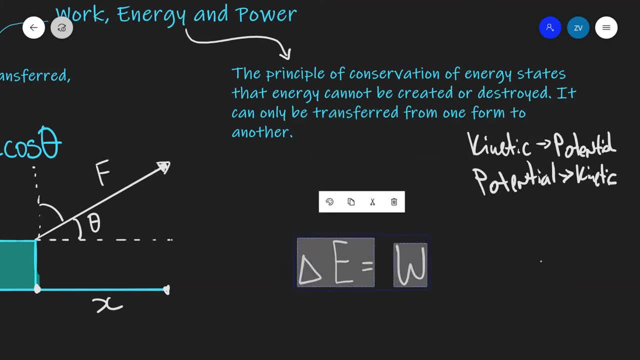 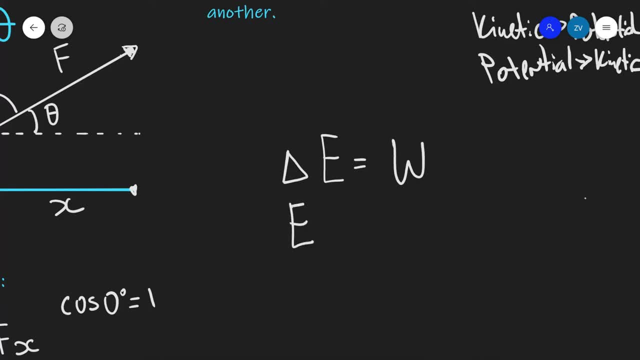 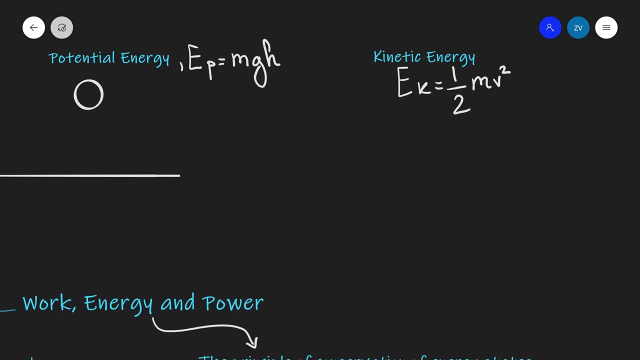 power of E to the power of E, to the power of E to the power of E2 minus E1, so let's call it E final minus E initial, and that will be equal to the work done on that system. Now that we have mentioned, 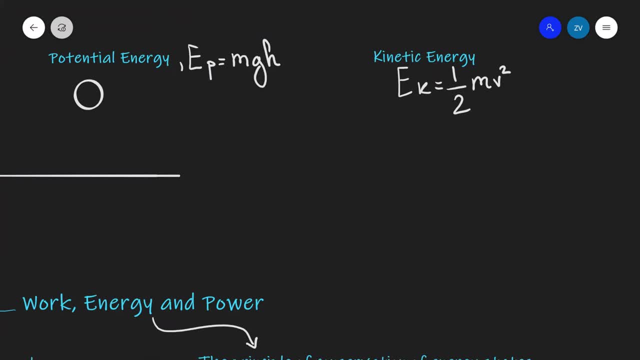 potential and kinetic energies as different types of energies. let's revise the equations for the two types of energies that we're familiar with and also derive them. Potential energy is given by mgh, where m is the mass of the object, g is the acceleration due to. 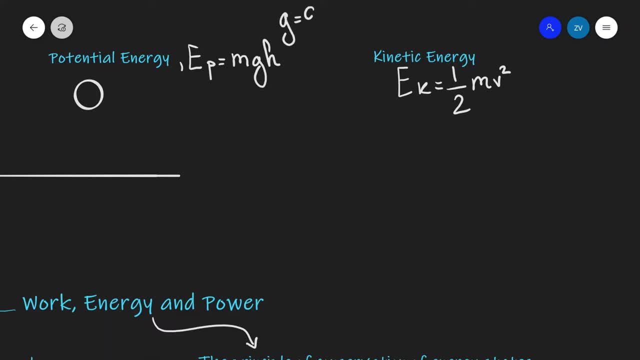 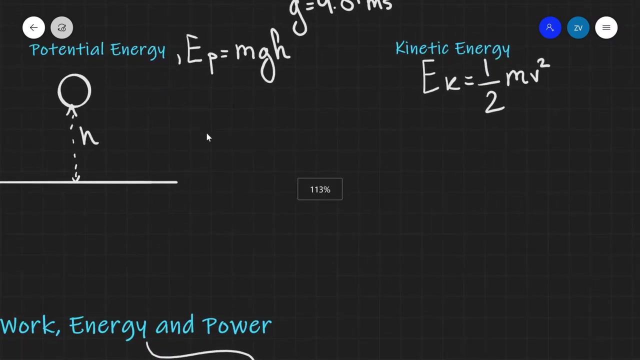 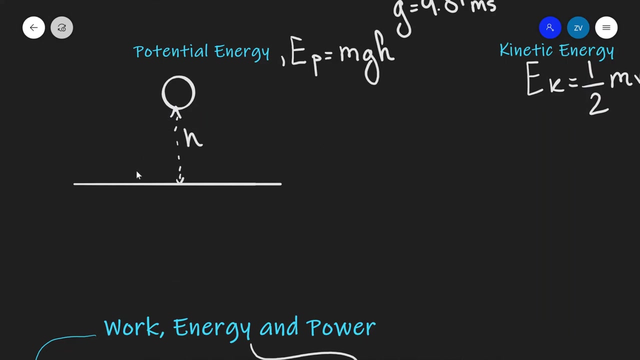 gravity on planet Earth, and that is equal to 9.81 meters per second squared, and h is the height within a gravitational field. Now let's focus on this first equation. Why is it that if we raise an object at a height h above the ground, or above a point that we take to be the zero point? 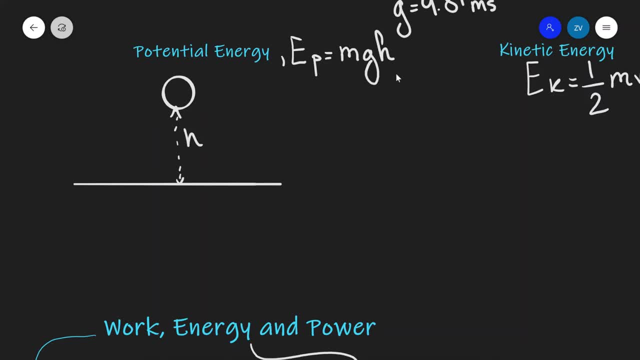 its potential energy, with respect to that point, is equal to mgh. Well, let's think about work done. The change of energy of that object will be equal to the work done. Now, whether we drop an object or whether we raise an object, the amount of work done will be. 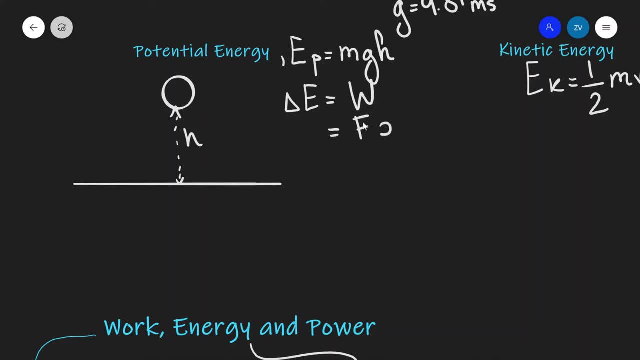 equal to the force times, the distance travelled, times, the angle, which is cosine beta. Now, in this case, the work done will have to be equal to the weight, because that really is the only force acting on this object, in the absence of air resistance and everything else. So work done. 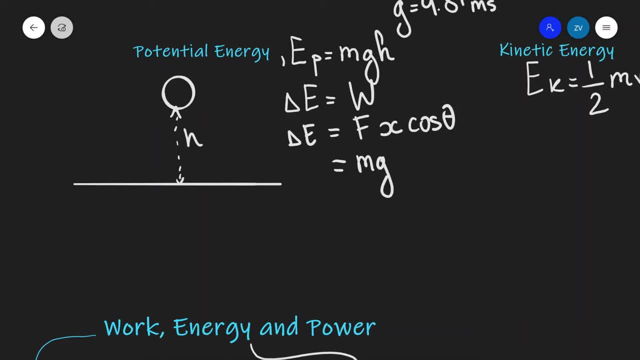 will be equal to mg times the distance travelled. Now, what about the weight that's travelled, which in this case is just the height, h and cosine of theta? Well, if we think about it, that's going to be zero, because the weight 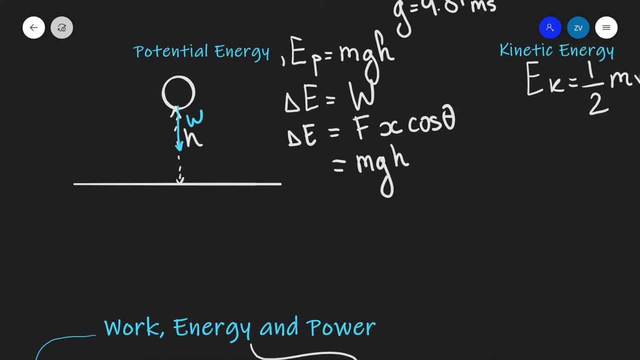 is acting along the same line as the height, as the distance travelled within the object. So in this case, cosine of theta will be- I'm going to write this over here: cosine of theta will be equal to one because the angle. 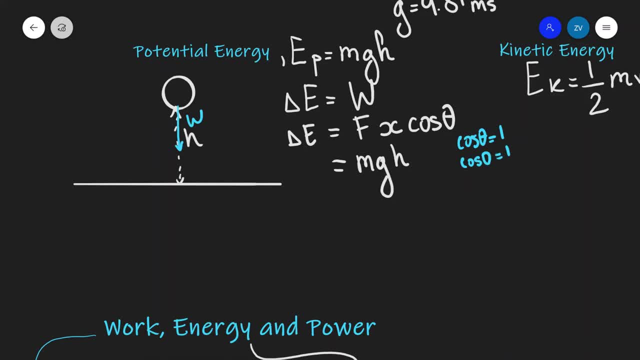 of zero degrees gives us cosine of zero, which is equal to one. So the change of energy of that object, delta E, is actually equal to mg h. So this means that if we were to raise an object at a height h in a gravitational field, its change of energy would be equal to mg h. 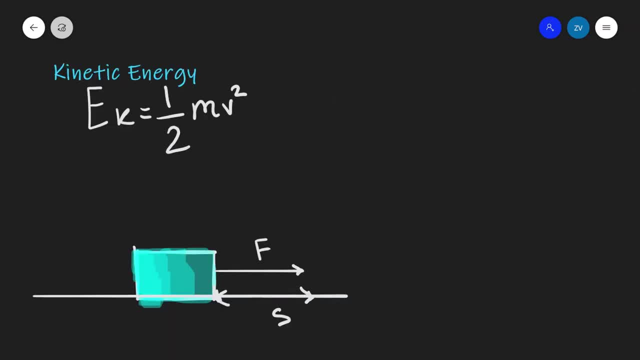 So now that we know why the equation for potential energy is true, let's see whether we can derive the equation for kinetic energy. It's absolutely amazing how these equations just come out of the fact that our change of energy- let's call that delta E- is equal to the work done. So let's 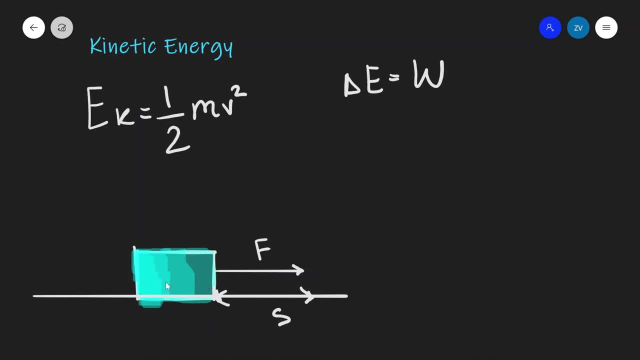 imagine that we have a box and we apply a force onto that box and we move it a distance s. At that point over here, let's say that the box starts moving with a final velocity v. So essentially what we're doing is we are moving this box to the right and it reaches a speed v. So a moment later, 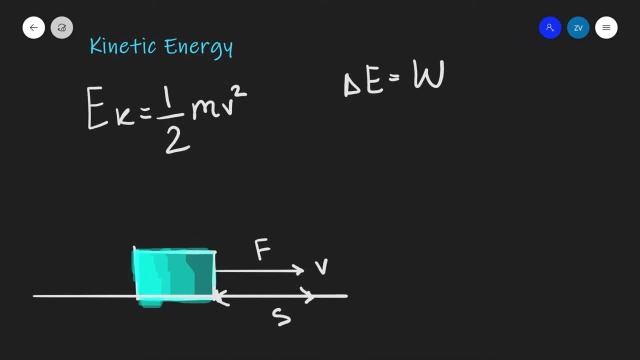 it's over here, moving at a speed v, Our change of energy of this object will be equal to the work done and, by definition, the change of energy would be equal to f cosine of theta. Now, once again, the force is parallel to the distance, so this means that our 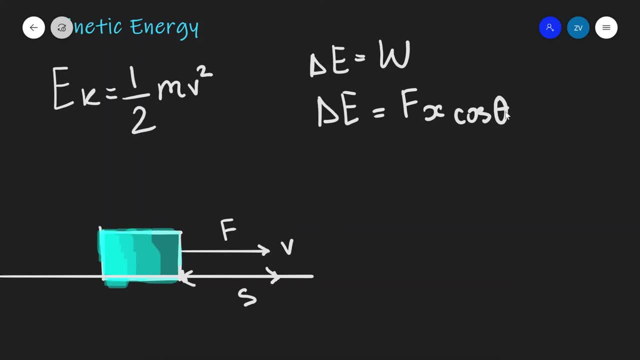 angle, theta will be equal to zero degrees, which means that cosine of zero will be equal to one, which means that delta E will be equal to the force times the distance, which I've called s over here, times one, but of course I'm not going to write out the one. Okay, well, let's. 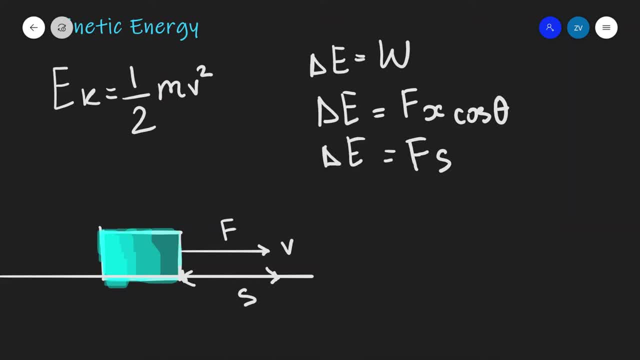 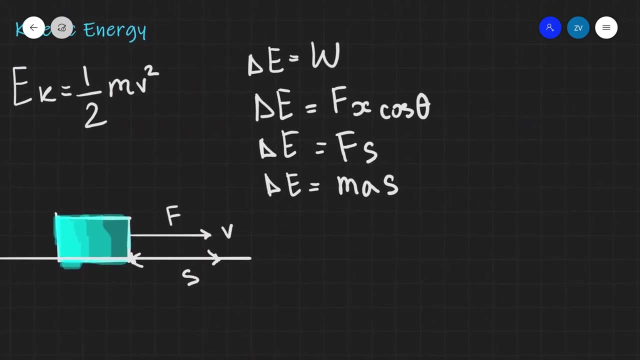 apply Newton's second law, which is that force is equal to mass times, acceleration in this case when the mass is constant. So delta E will give us m a times distance travelled. Okay, we're almost there. Now, because we're dealing with acceleration, let's also think: 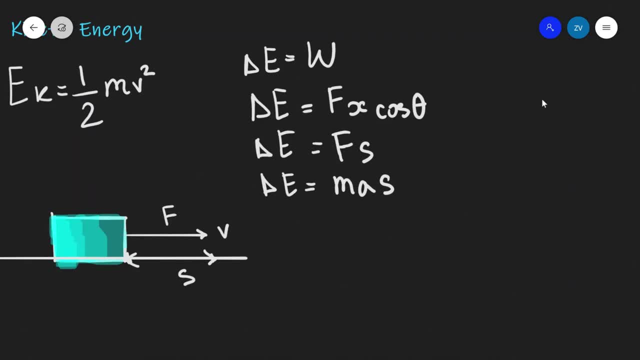 about the suvat equations. We know the suvat equation that v squared is equal to u squared plus 2 a s. and let's say that this block has been accelerated from point one to point two and point one is addressed. so let's say that this block has been accelerated from point one to point two and point one is addressed. so 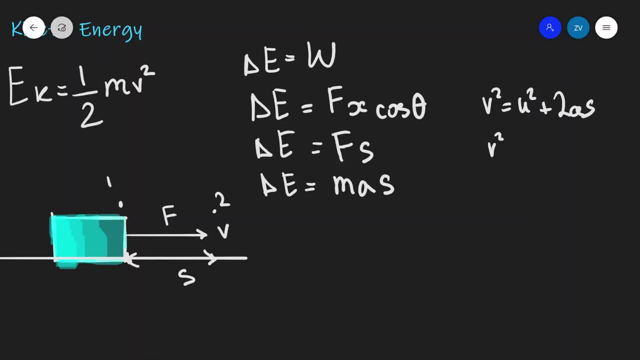 we know that this block has been accelerated from point one to point two and point one is addressed, so u is going to be zero. So this equation just becomes: v squared is equal to 2 a s. Well, notice something: I have a s over here. I have a s over here as well. 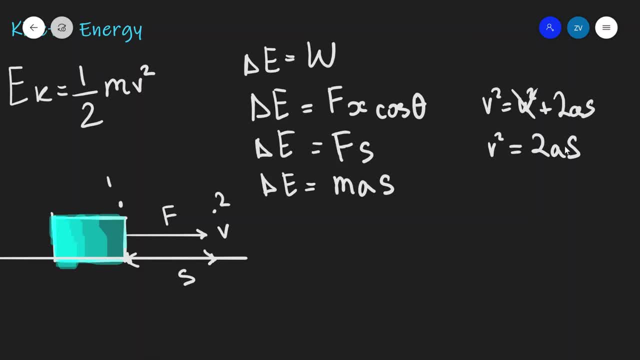 so this means that I can directly rearrange for essentially a s. So I'm going to say that a s is equal to v squared divided by two, and what I'm going to do is I will essentially plug in this expression because that's equal to a s, that's going to be equal to 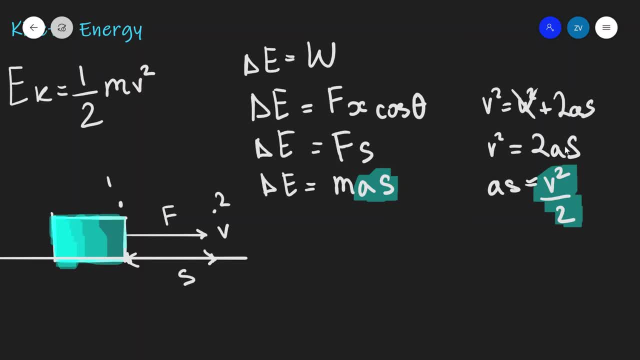 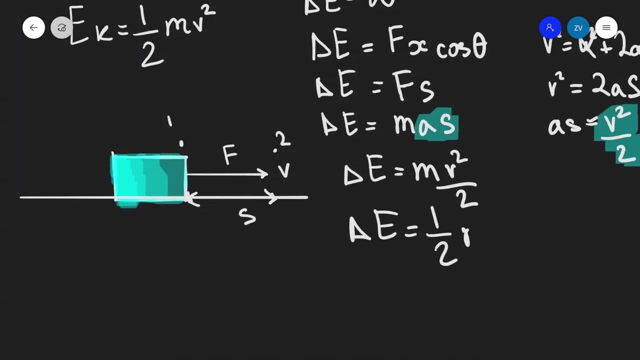 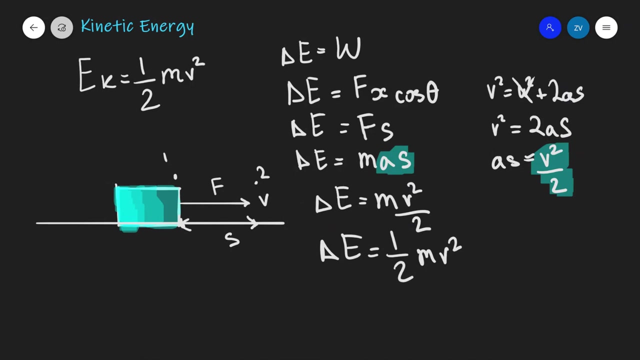 to this guy over here, which gives us that the change of energy delta e will be equal to m times v squared over 2.. well, look at this. this is actually mathematically identical to delta. e is equal to a half m v squared. we have managed to derive the formula for kinetic energy from first. 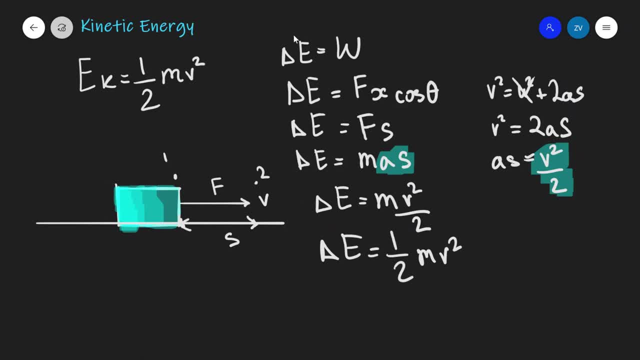 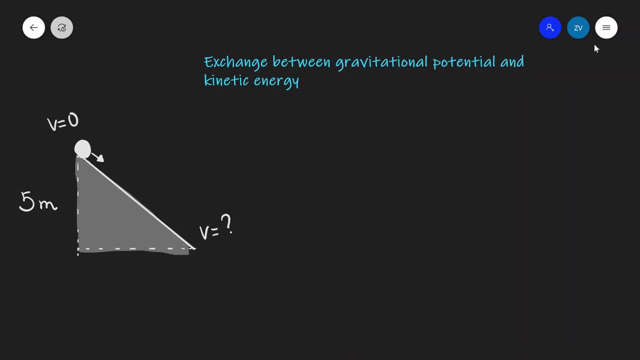 principles, using the fact that our change of energy is equal to the work done. let's have a look at the exchange between gravitational potential and kinetic energy in order to do so. let's imagine we have a ball which is on the top of a hill and we roll this ball down and it reaches some speed. 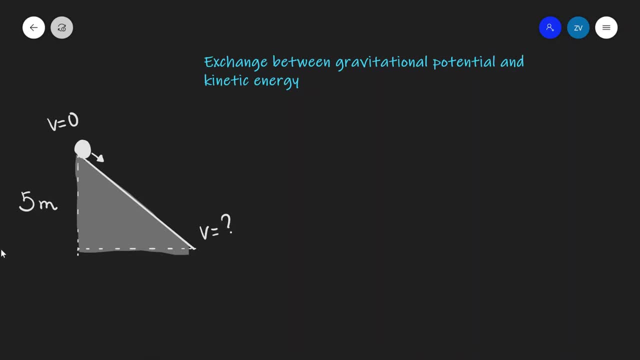 v. now, what will that speed actually be? the height of the hill. the vertical height of the hill is five meters, and that's this is really important. the ball will have zero initial velocity. in order to figure out the final speed, we're going to use the principle of conservation of energy initially, the ball only. 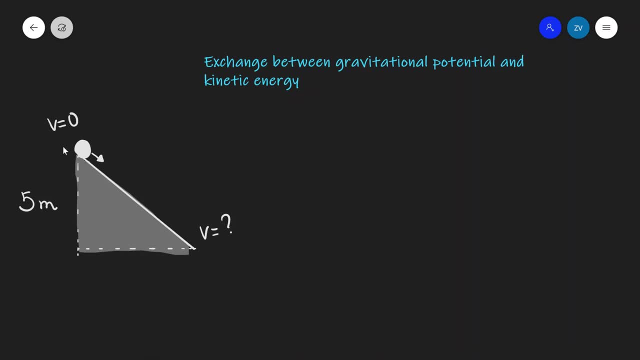 has potential energy because it is at rest at the top of this plane. so initially our energy is equal to m, g, h. now, at the bottom of the hill, all of that energy is converted to kinetic energy. so the total energy after the event, after the ball is rolled down the hill, will be a half mv squared. notice that. 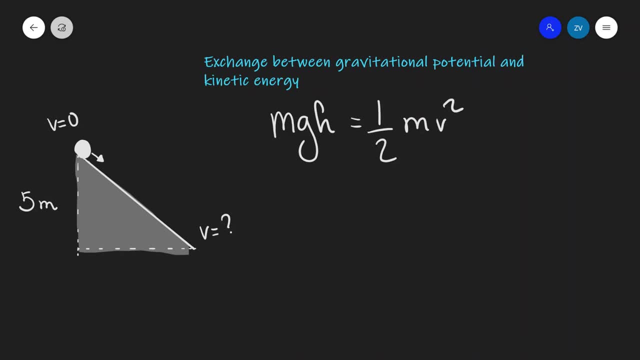 the final speed will be independent of the mass of the ball, because the masses are just going to cancel out, just rearranging for the speed we're going to get that v squared is equal to 2gh, which of course means that v will be equal to the square root of 2gh, which is equal to the square root of. 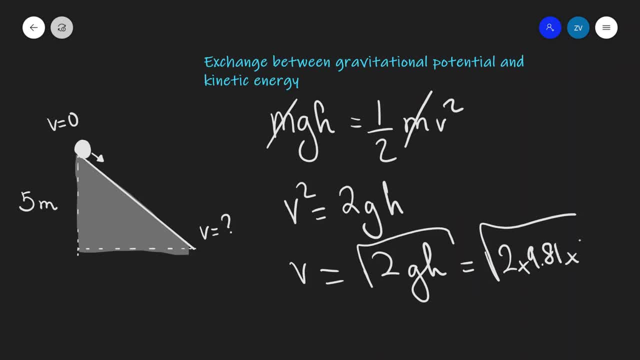 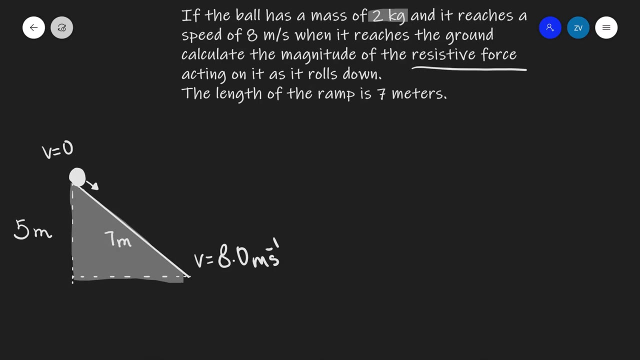 2 times 9.81 times 5, and if we put that into a calculator, we're going to get about 9.9 meters per second. now, the previous problem involved absolutely no resistive forces, so no friction, no air resistance. let's have a loka-aei. 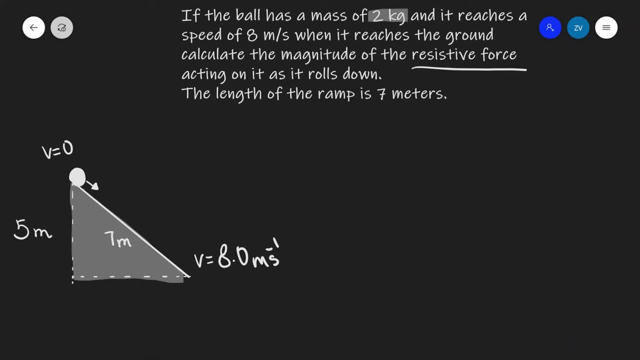 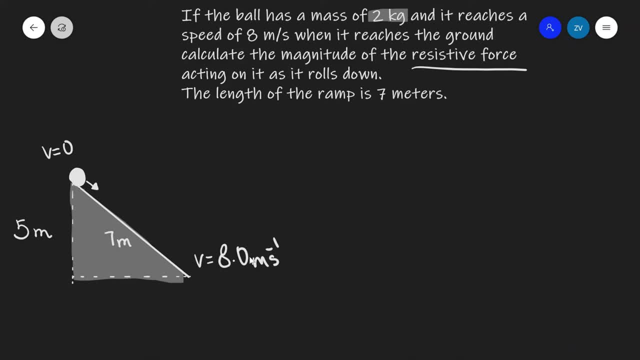 reaches a speed of 8 meters per second at the bottom of the hill, and if the length of the ramp is 7 meters, let's see whether we can calculate the magnitude of the resistive force. In order to tackle this problem, we're going to use the fact that the change of energy is equal to the 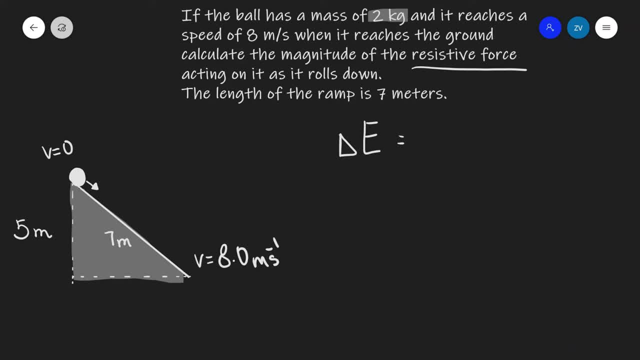 amount of work that's been done on this ball. So delta E is going to be equal to the work done Now, our change in energy. delta E will be equal to the potential energy, because at this point we only have potential energy. so let's just write down: mgh, take away a half mv squared, because 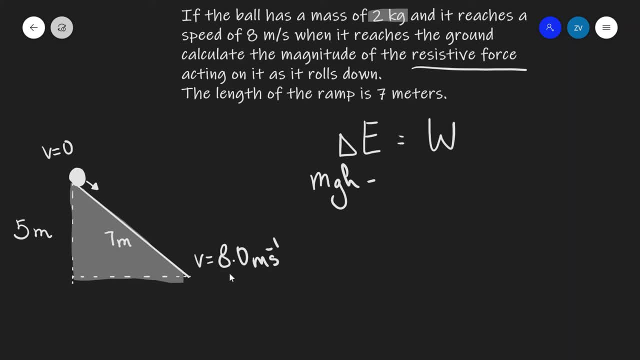 that's the energy in this position over here. this is our change in energy. Let's say, if here we had 10 joules and here we had- I don't know- let's say 8 joules, then we know that 2 joules have been lost to resistive forces. so take away a half mv squared, This will be equal to the work. 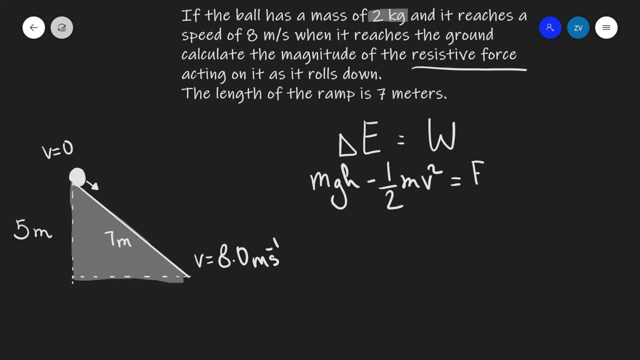 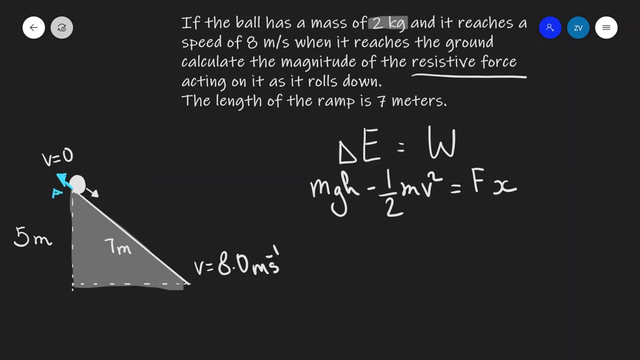 done, which is equal to the magnitude of the force times the displacement. Notice that for work done I'm not using fx, cos theta, because the resistive force will be acting along the same plane. along here I can just show you the resistive forces. Let's say that this is F and the angle between the force F here and the displacement. 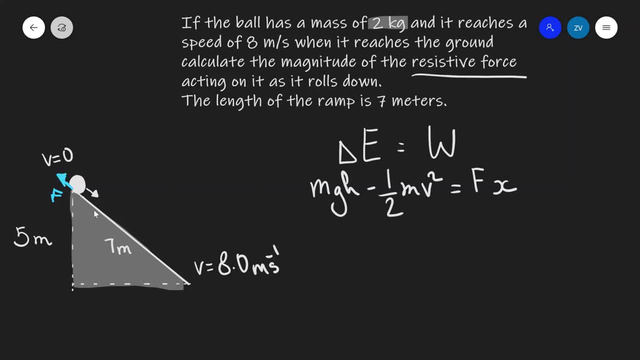 is actually zero because the resistive force is along this plane. Okay, well, let's input some numbers and be able to essentially rearrange for the force F. So our mass of the ball is two kilograms, so it's going to be two times 9.81 times the height, which is five. take away a half times. 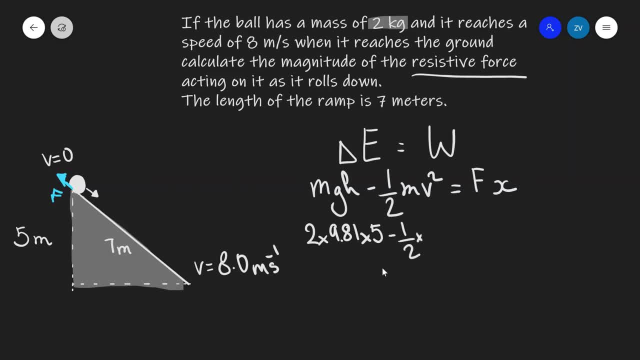 the mass of the ball, which is two kilograms, times V squared, which is the speed at the end, which is 8.0 squared, And this will be equal to the magnitude of the force, which is what we're looking for, And our distance traveled by. 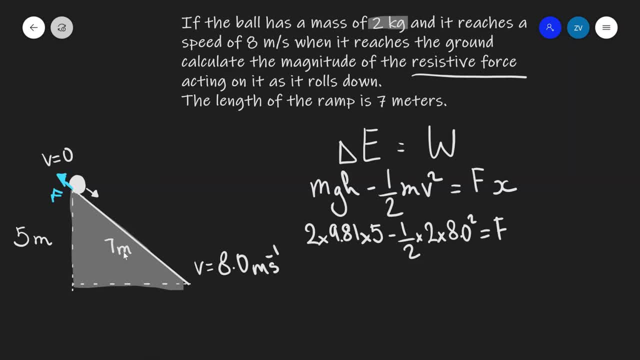 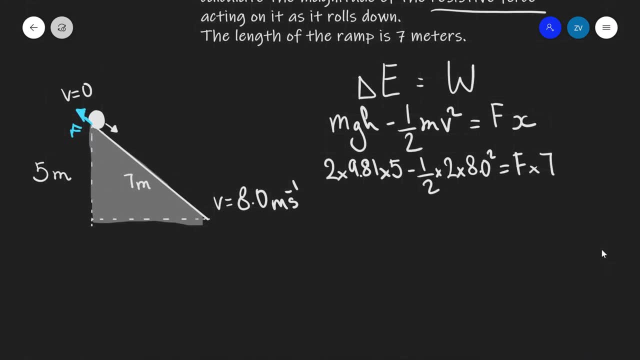 the ball is the length of the ramp, which is seven meters, So it's going to be F times seven. We put this left-hand side of the equation in a calculator, we get 34.1.. So that's 34.1. 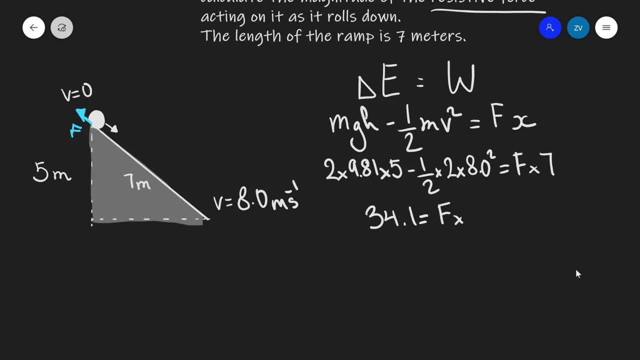 will be equal to the force times seven. And just finally, managing for the average resistive force, We get that the average resistive force is equal to 34.1 divided by seven, which in turn equals about 4.9 newtons. 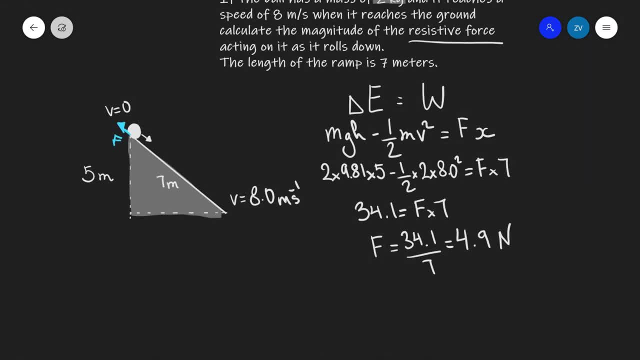 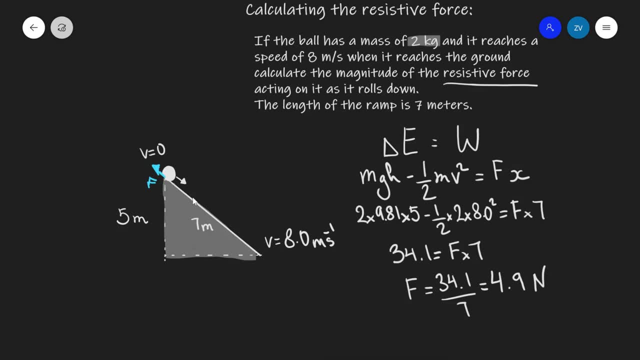 So this is the amount, the average amount of resistive force which is acting on this ball as it's traveling down the plane. Now remember, guys, what we're actually revising today is what the moment dominates of the mass factor. If we look at this literature, if we look at the momentum data, we can place the angle of the wall in that direction. If we look at this, you don't get a lot of�리 far. So one guideline is that the left hand side of the ball is velocity. the imaginableness of the won is at 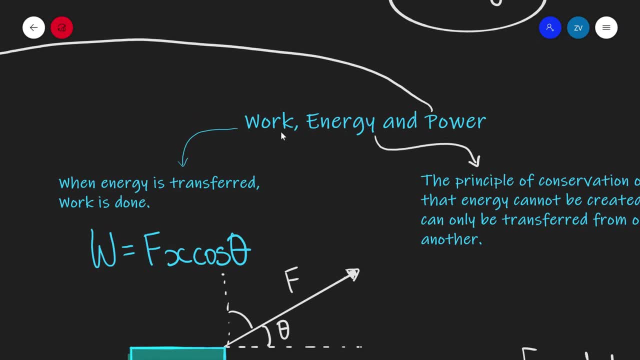 all one guideline. So we said we can't always say the을害ISM, that's the right hand side of the machine, but you can see, today is work, energy and power. So we've done quite a bit about work, quite a bit about energy. 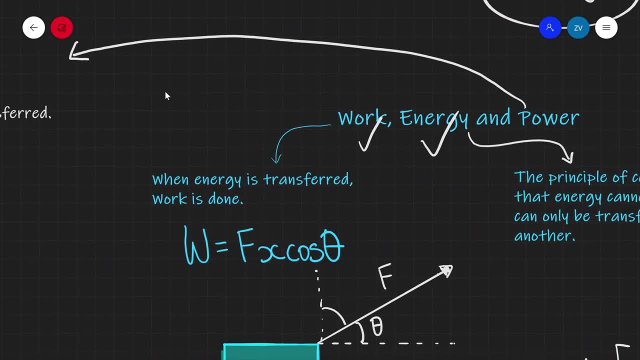 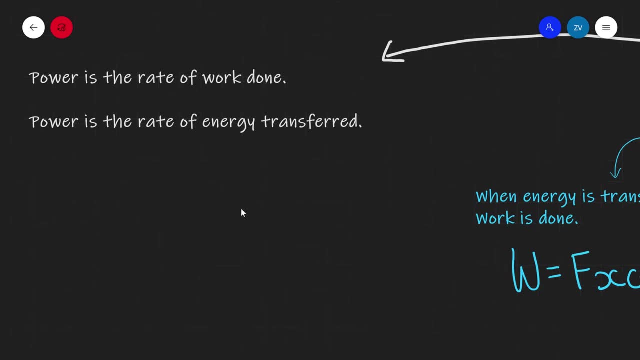 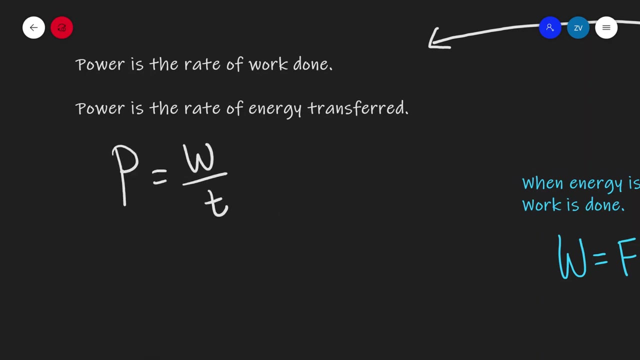 Now let's focus a little bit about the power. Now, what is power? Remember, power is the rate of work done or the rate of energy transferred. Mathematically, the equation for power is w divided by t. Anytime we're dividing by time, essentially it's the rate of change of a. 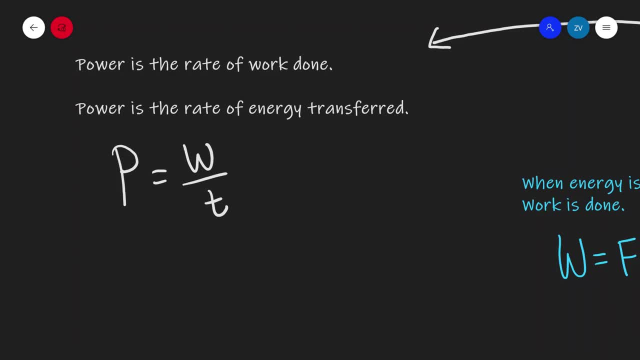 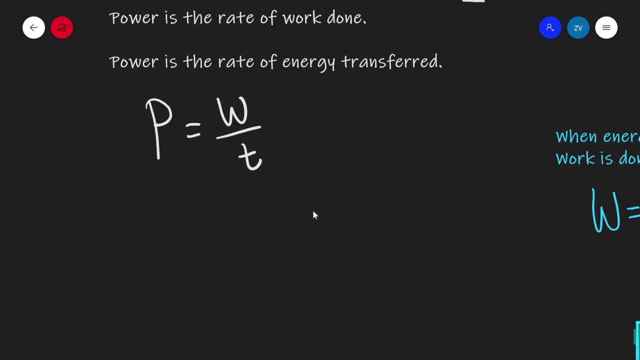 particular quantity Because work done is given by force times, distance times the cosine of the angle. let's imagine the force is parallel to the direction of motion. work done is just equal to f times x. Another way of writing power would be f times x divided by t. Well, let's have a look at. 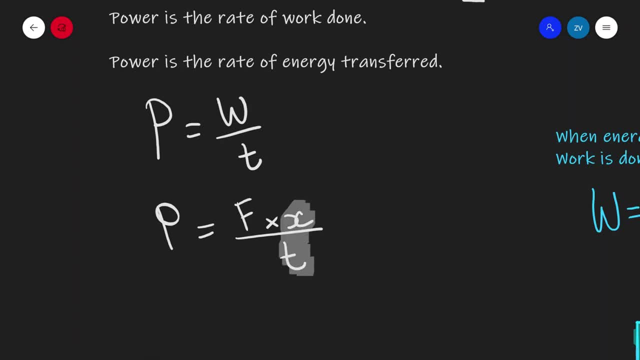 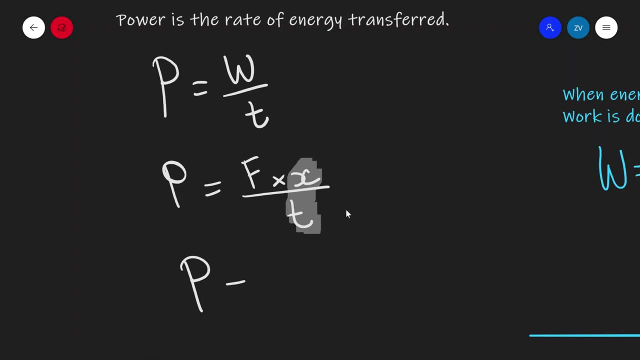 this x over t distance divided by time, This is actually the speed. So another equation for power is that power is equal to the force times the velocity. One final equation that we need to revise is the mechanical efficiency of a system. We can 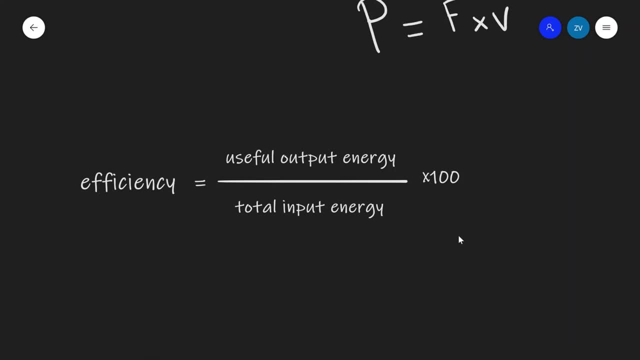 actually really easily calculate the efficiency. All we need to know is the total useful output energy. So how much of the total energy has been used to do useful work and what was the total input energy? We divide the two numbers, we multiply by 100, and we're going to get 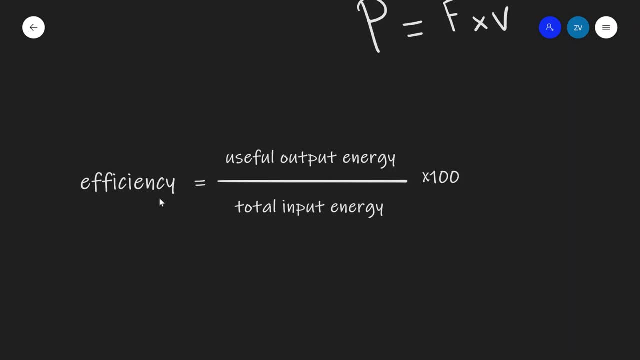 the percentage efficiency of our system. Of course, this equation will give us a result which will be in terms of percents. Okay, folks, so this was a revision lesson on work, energy and power. Hopefully you found this useful. Thank you very much for watching and I'm going. to see you guys in the next video.